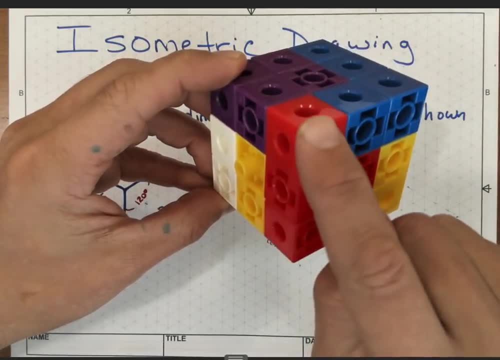 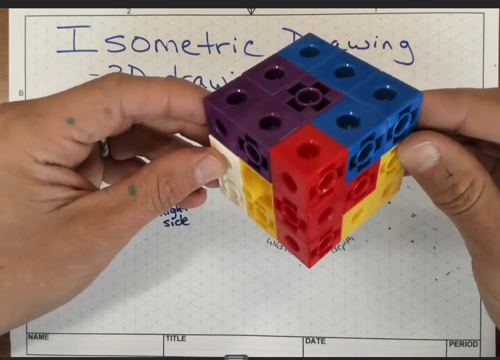 I would need to position it so that this corner, where the front, the right and the top all meet, is pointing straight at you, And I need to get that right. So I'm going to rotate the right amount of orientation this way. 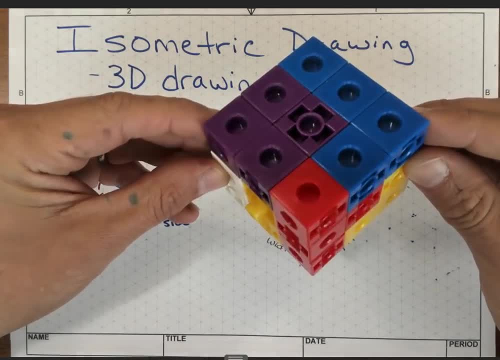 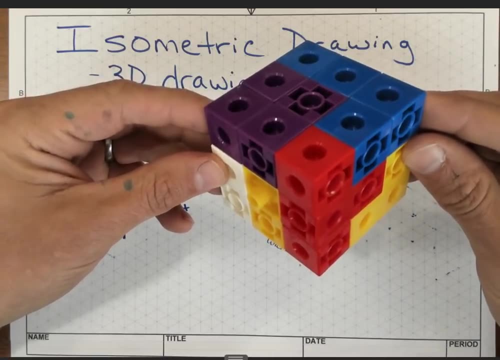 You can see the front and the right are kind of fading away here to only see the top, And if I rotate this way, the top is going to fade away. Now, if you look at this and we look at the edges where the front and the top meet, 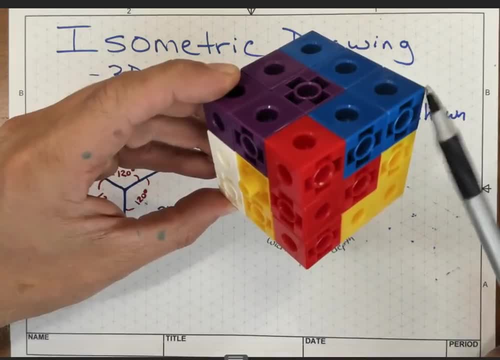 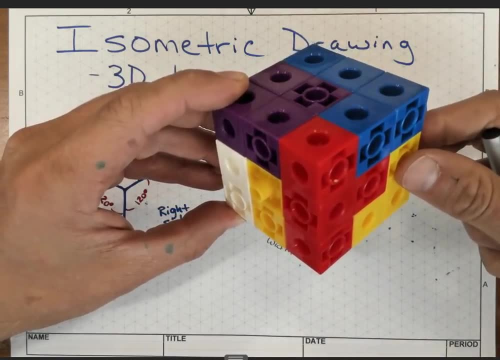 okay, so this edge right here, and we look at the edge where the front and the right side meet, right here those edges form a letter of the alphabet and it is the letter Y. Now we have special graph paper used to draw isometric drawings. 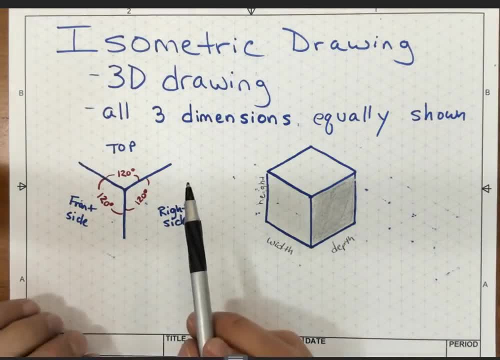 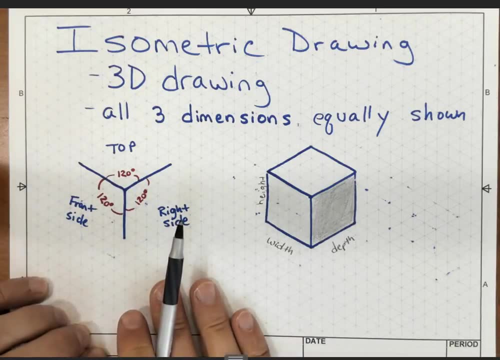 It's called isometric graph paper And if you look at the lines and we bring together: okay, the vertical line, you should always have a vertical line with isometric drawings- okay, with the other two directions, and you form the letter Y. the angle between these lines is all 120 degrees. 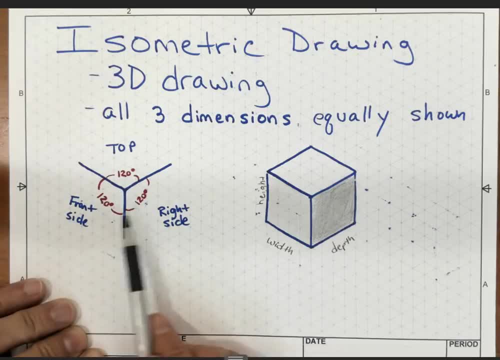 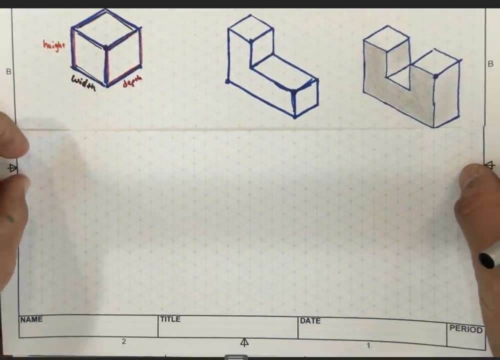 So, because they're all equal. that is why we're presenting all of them. We're presenting all of these dimensions of width, depth and height equally, all right. So let's try to do some examples real quick. You can do them with me, but that is what an isometric drawing is. 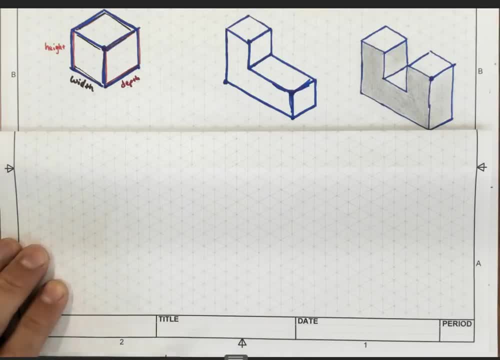 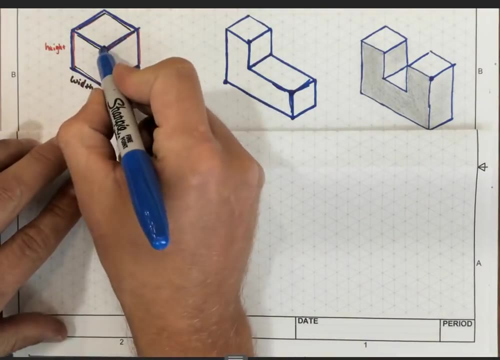 Okay, first I'd like you guys to try a cube. Go ahead and pause the video right now and give it a shot. Okay, hopefully you gave it a shot. Let's do it in Sharpie real quick. One suggestion is to pick out a corner to start with. 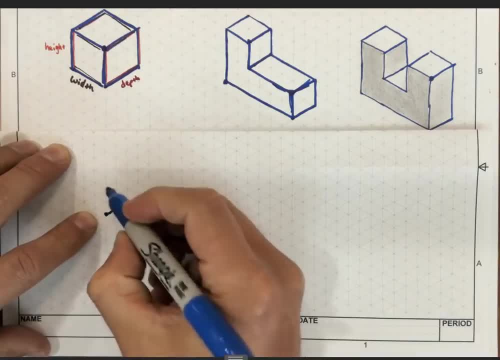 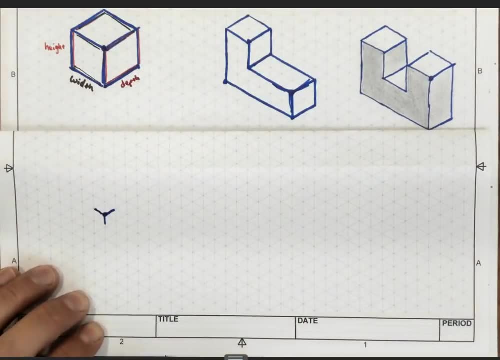 And so how about I use this corner, and we talked about the Y, and you can even just go one segment by one, by one, basically where these plants come together and start to see a corner, And then from there you can start to look at how many units. 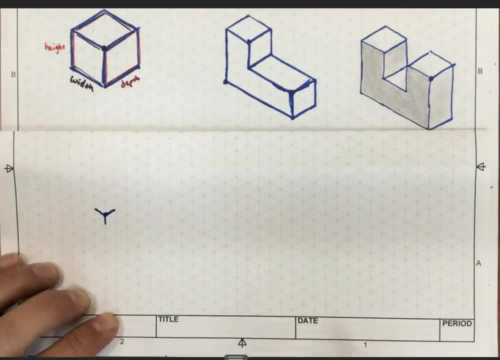 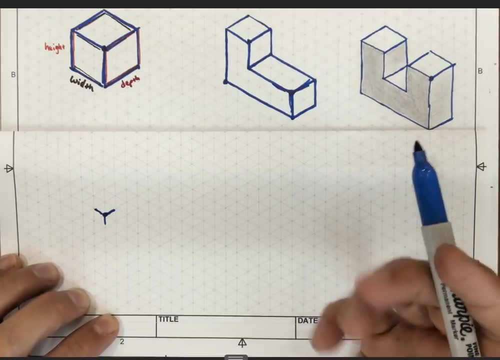 what are the dimensions and rebuild your drawing. Right now we're just going to practice drawing some isometric drawings of objects we've already seen. We're probably just copying them to get practice. But this is a three by three by three cube. 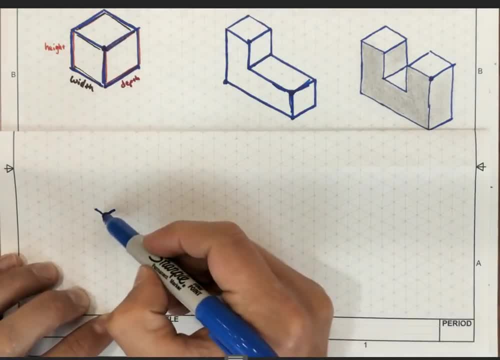 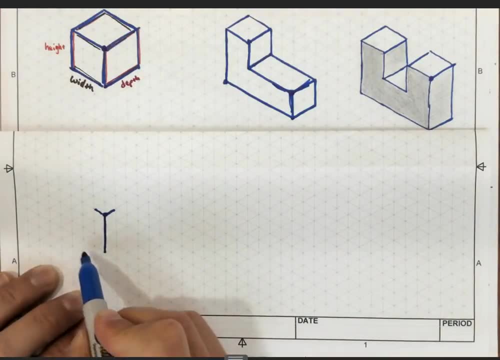 And I'm starting right here. So I'm going to focus on this front face right here, where this is the top right corner, So it's going to be three units tall. So the vertical line gives me my height And then these diagonal lines going this direction give me the width. 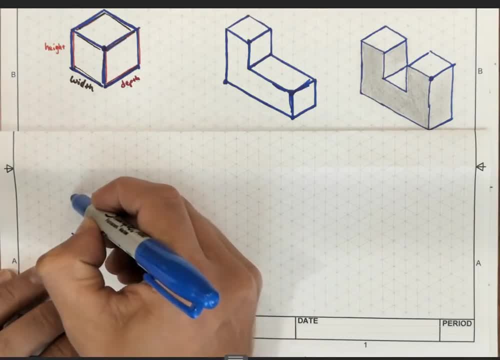 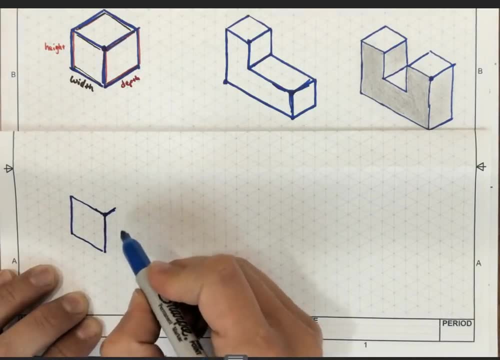 So it's three by three. So I'm going to make it right here: three by three and a height of three. So I drew one face. Now how about I do the right face? It's going to be underneath here When I draw the lines. this direction, kind of the up and right direction. 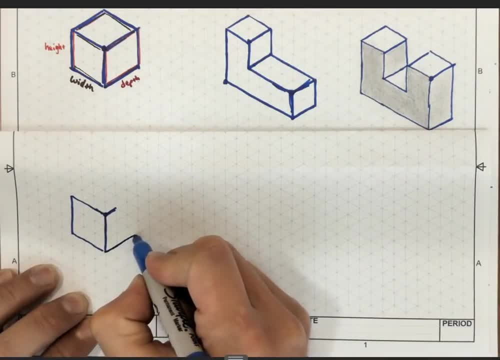 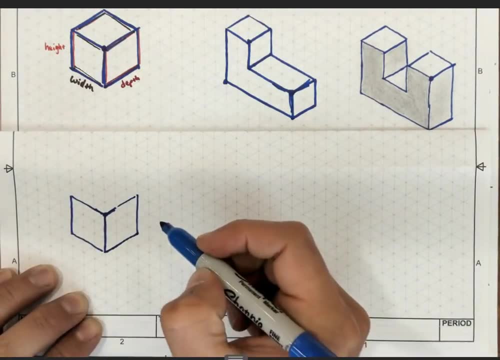 that's allowing me to see depth, So it's three units deep as well. So there's depth and again the vertical lines are my height. So there's the front face, the right face and then the top. Now the top has depth, so I need to show the depth here. 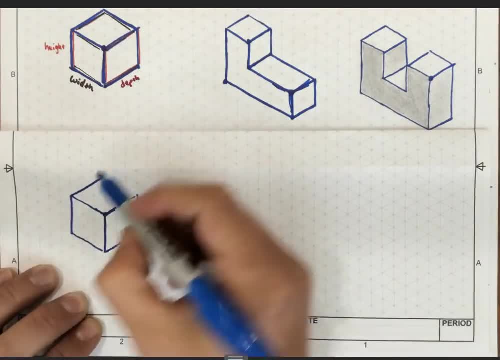 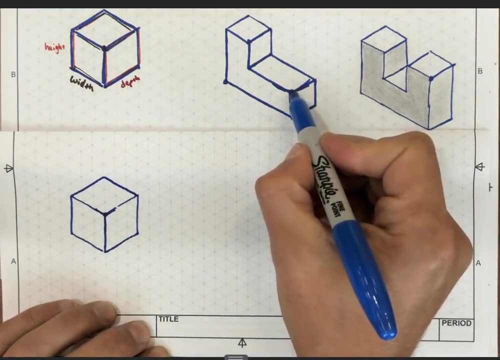 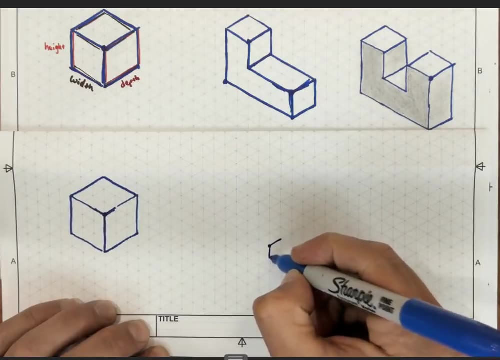 And it also has width. The top is width and depth. And there you go, Let's try this one. I'm going to start with this corner right here. So I'll find a point on my graph paper And I'm just going to give myself kind of a one by one, by one. 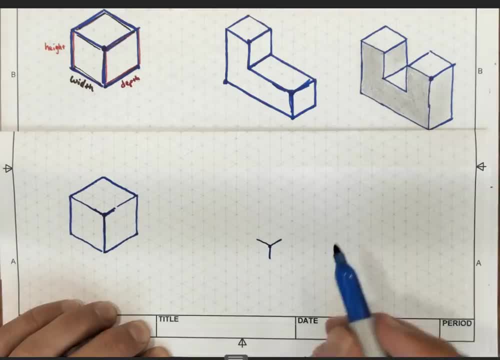 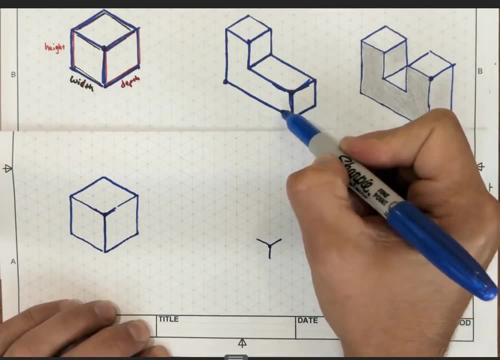 just to start showing those different planes And I would focus on one face at a time. So I'm going to do this L-shaped face Starting at that corner. I'm basically going to trace my way around. So the front face has width. 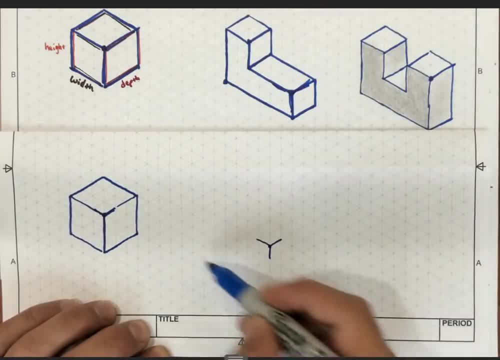 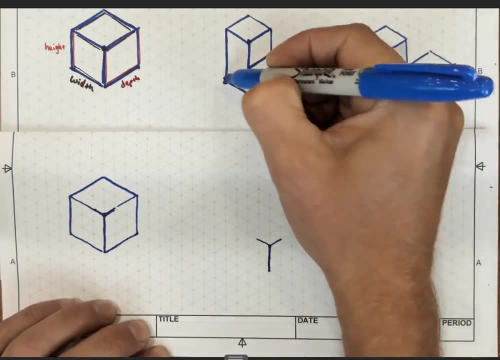 So I'm going in this direction And it has height. I won't see depth, So I'm going to be working in this direction and vertically. So right here it looks like I'm two units tall And if I count this out it's six units. 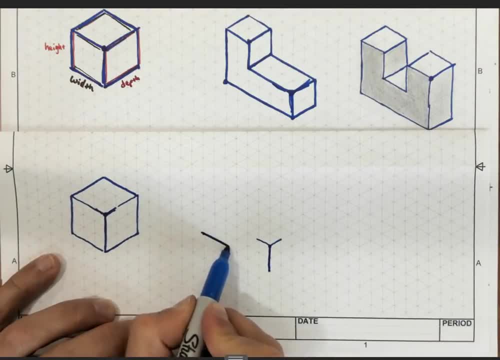 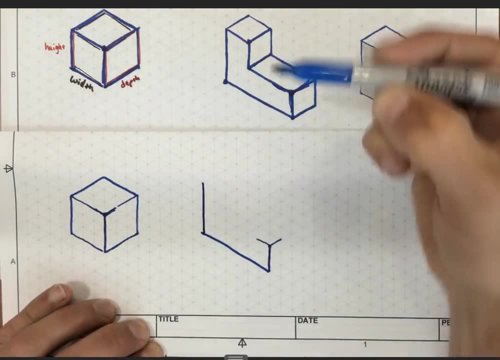 So let's see two, four, six. So it's going to go all the way to here And on the back the height is four units. So two, four, And then the width of this bump out is two units. 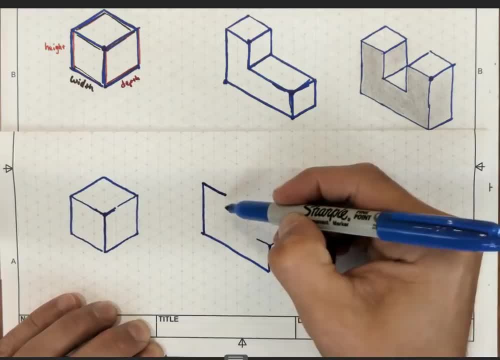 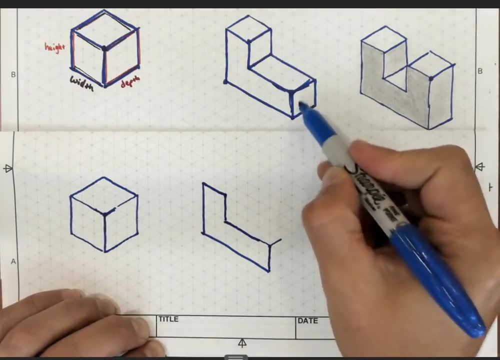 So again, width is this way, Height is this way: A height of two there And then a width of four. That should take me all the way back. All right, now I'll focus on these other faces. This face right here, it's a vertical plane. 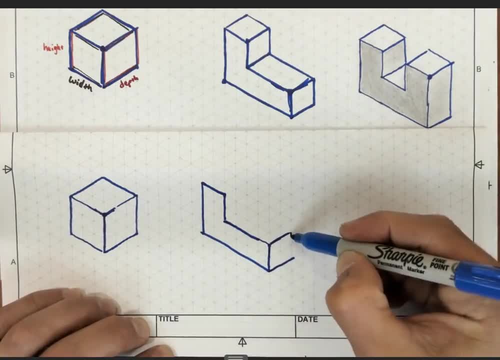 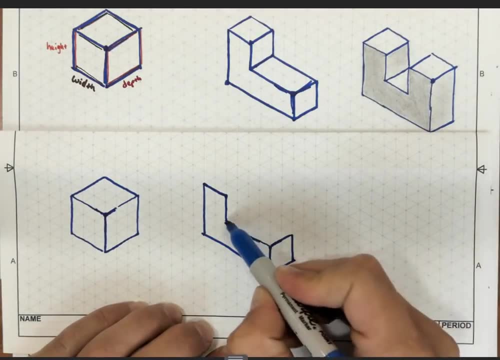 It has a depth of two and a height of two. So there's my depth of two and a height of two. Now I have a horizontal top face. It has a depth of two units already defined right here. I just need the other edge to show depth of two. 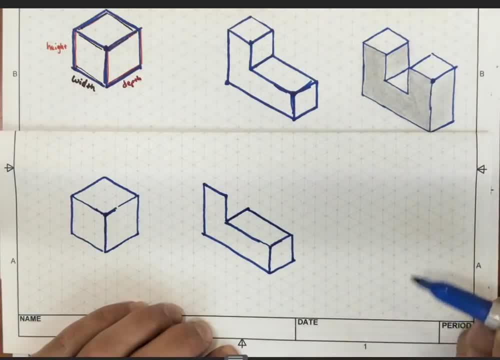 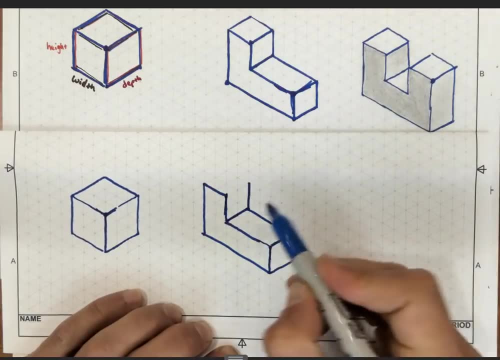 And it has the width of four parallel to that, And then I have another vertical plane. This object turns up. It has a height of two, Height of two- right here I already had- And then this depth of two And then the top. 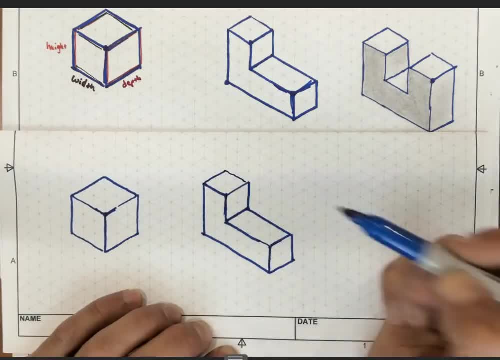 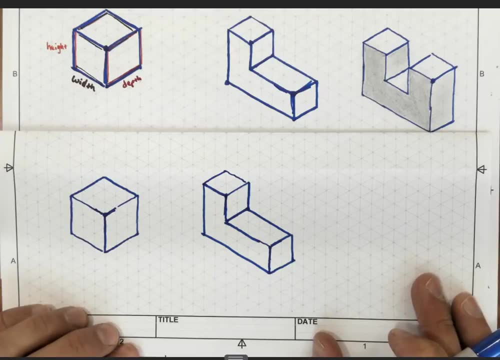 So a width of two, a depth of two, and there we go, All right, and there's another one to try. You can pause the video here and take a second and try that one. Okay, hopefully you tried it. Let me draw it. 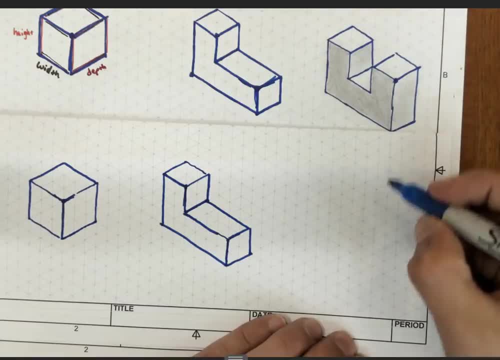 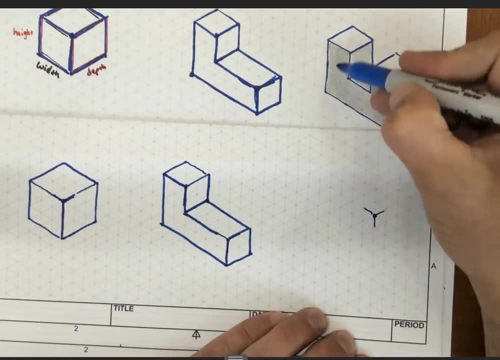 So again, I'm going to identify a corner. to start with, I'm going to use this one- You might have seen that dot- And again I'll just give myself a little line to start these- And I'm going to focus on this kind of U-shaped face. 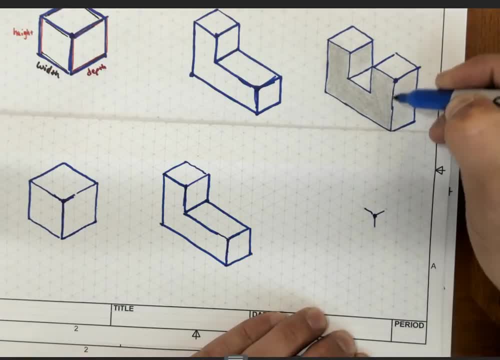 All right, it looks like I have a height of four units here from that corner, So I'm going to kind of work my way around that face. So I have height and width to show. Width's going this way, Height's going this way. 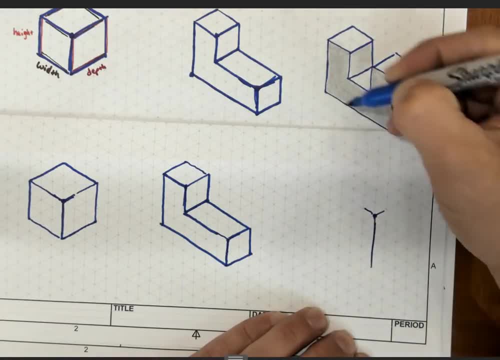 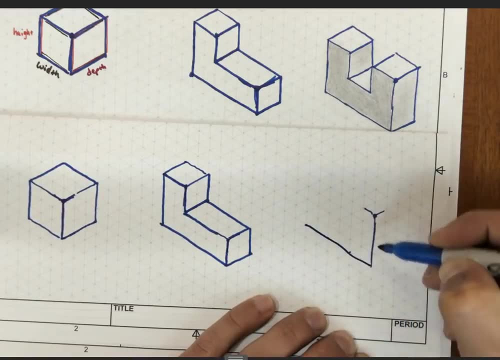 So height of four. Let's see two, four. right here I have an overall width of six. So width is this way. Let's see there's two, four, six. I have a height of four. again on the back, 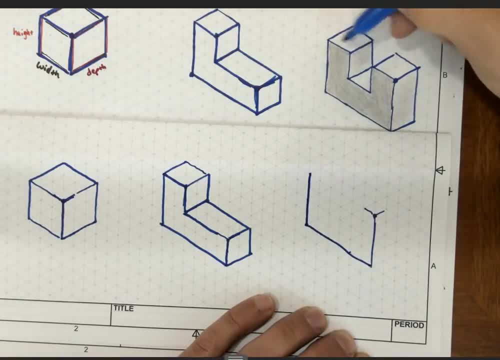 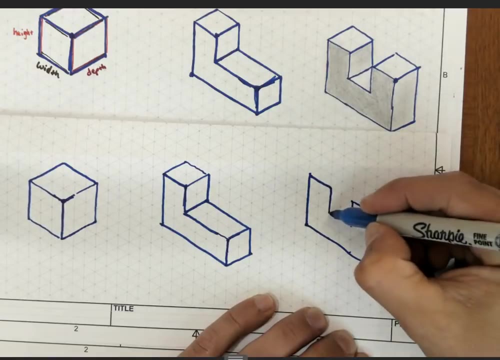 So there's two, four. Now this bump out on top has a width of two, This has a width of two, And then those bump outs have a height of two. The overall height's four, but those are two units tall. So do that. 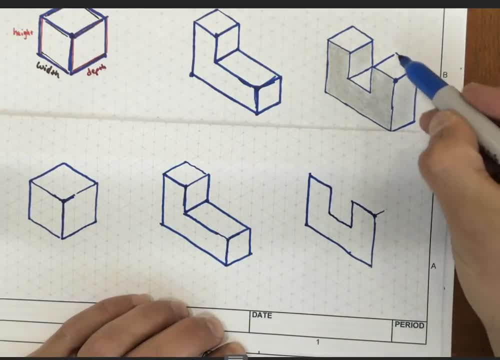 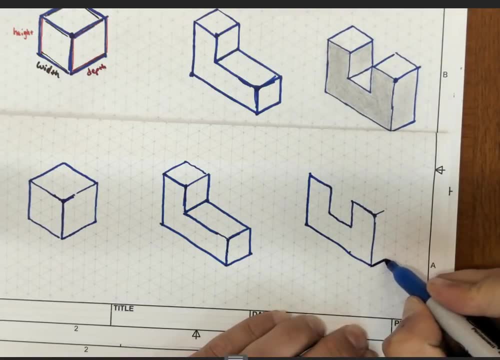 And there's my U. Okay, so now I'll take some of these other planes, these other faces that I can see. So this right face here has a depth of two and a height of four. So here's my depth of one, two. 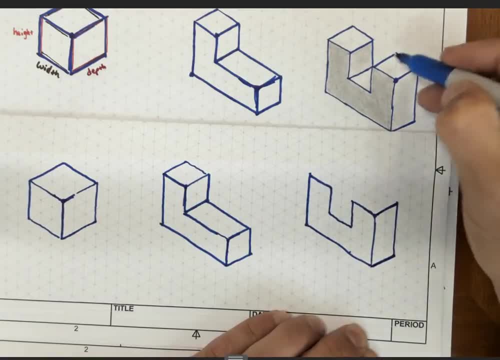 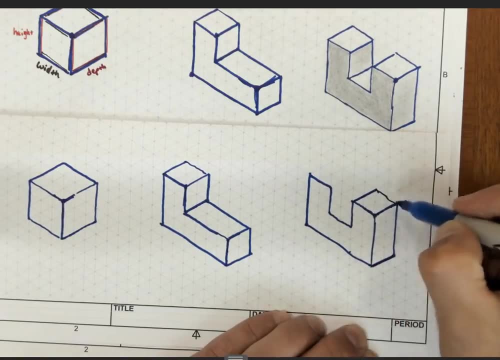 And a height of four. And then on top, this top face has a width of two and a depth of two. So there's my width, My width, Those are my depths. Same thing on the back there. Let's just do that one. 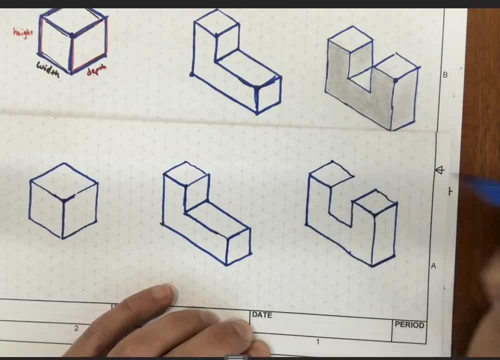 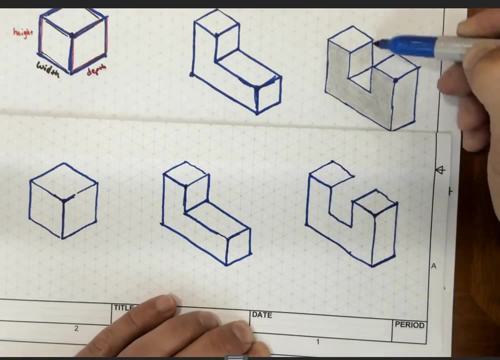 So a depth of two again, And I need to add some extra lines in to understand this. So this vertical face, this edge here, has a height of two. So I'm going to come down two units And that kind of runs into that. 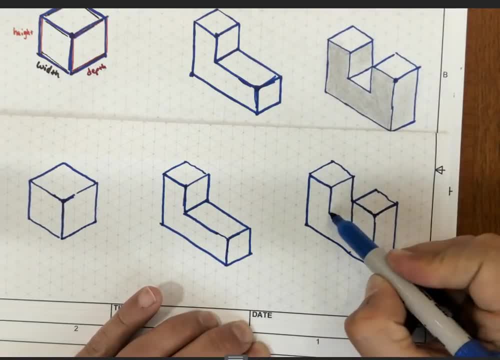 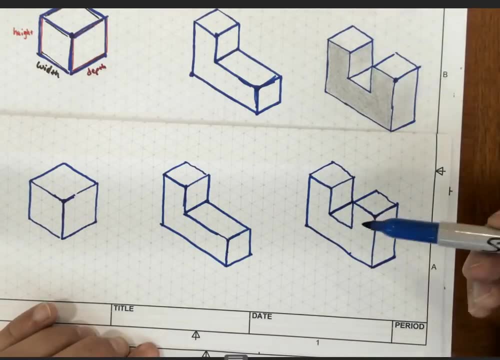 And it has a depth of two. I need to show from this corner to this right here. So I need to show that crease, that edge where those two planes meet. And one of the things you'll notice if you compare these two is that your eye can get a little confused sometimes as you're looking in here. 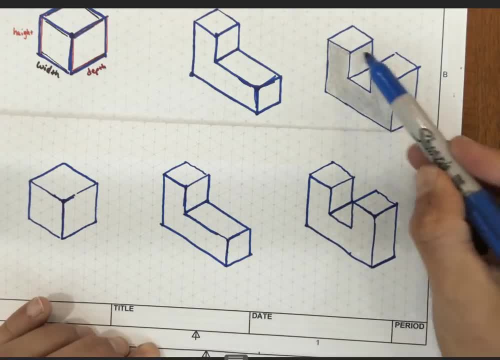 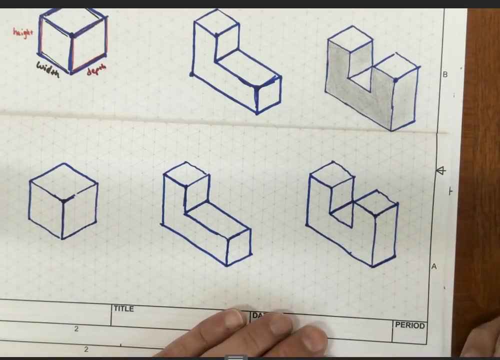 And so I have tried to help your eye see the three dimension by using what's called tonal shading. Okay, If you imagine a light source, Kind of up above and behind the object, maybe a little to the right, So kind of picture the sun. 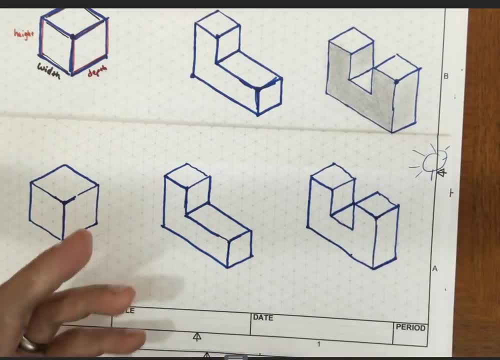 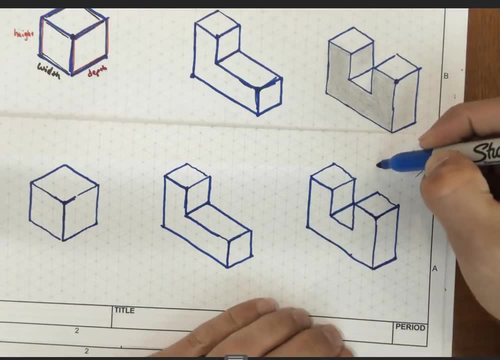 A single light source shining. We're going to get some faces that get more light than others. Some are going to be darker, more in the shadow, And so we think of faces that are facing up, faces that are facing to the right and faces that are facing out to the front. 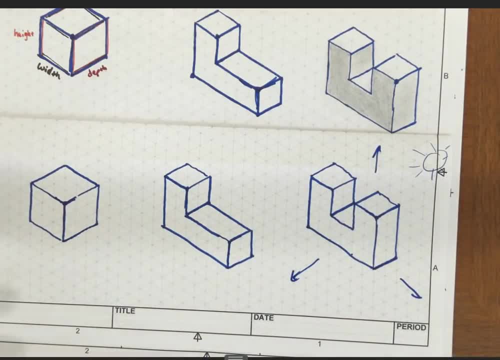 And we determine which ones are going to get more light and less light. So I'm going to say I'll kind of rank them one, two or three. One's going to be the most light, Three's going to be the least amount of light. 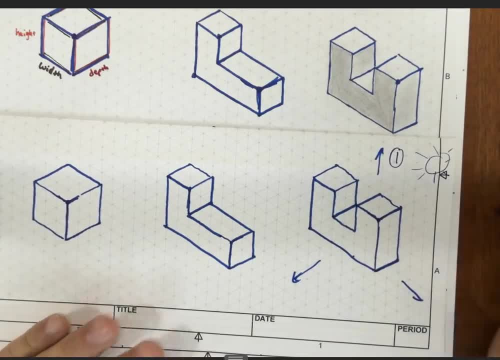 So, if the sun is up above, I'm going to say that the faces pointing up are going to get the most amount of light, And I'm thinking of this light source being up high, but also a little to the back, And so I think of the front face as being the darkest. 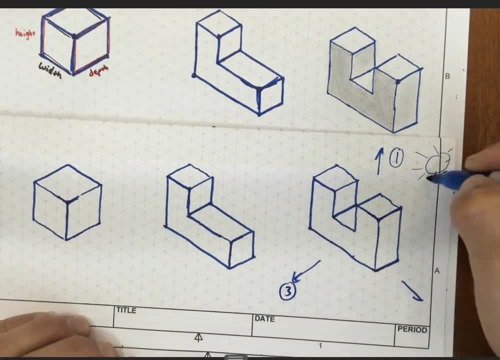 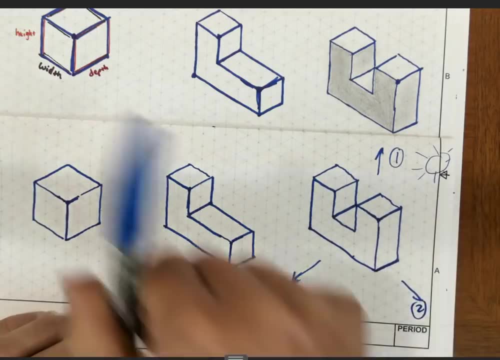 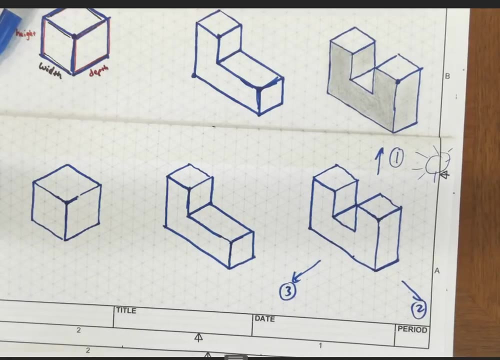 So I'm going to put a three there for the darkest And then two. I'll think more light can wrap around the sides and get the sides lit up a little bit better than the front. So I'll make that a two. I'm going to shade these surfaces accordingly. 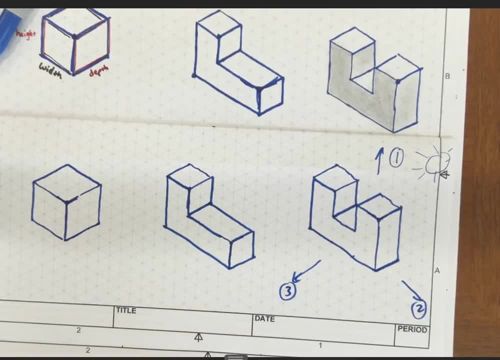 So anything that is, Let me grab a pencil, Pencil's a little easier to do some shading with. Anything that's the brightest, I just won't even shade at all, I'll just leave it unshaded. So my lighter shaded, but lightly shaded, the twos are anything that's facing out in this direction.